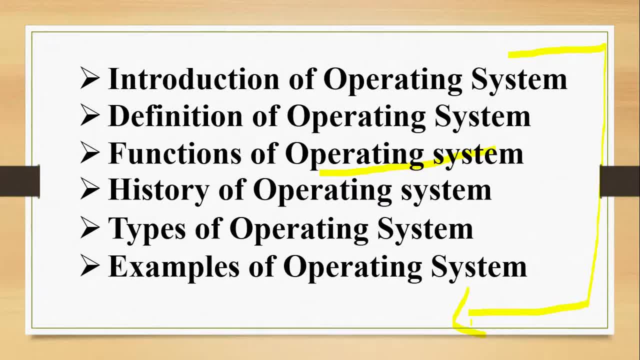 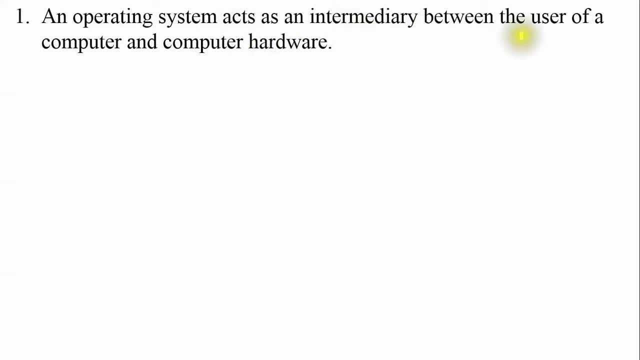 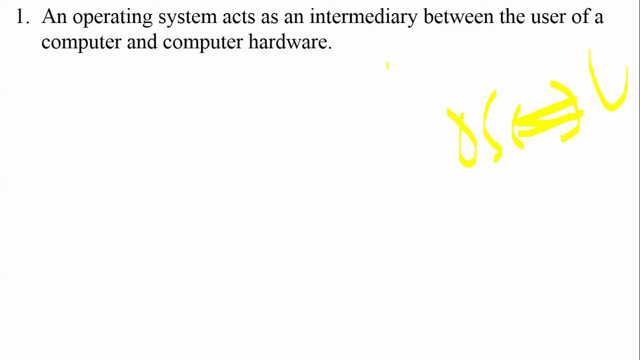 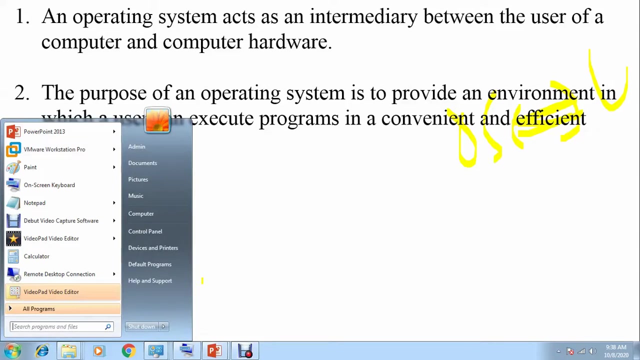 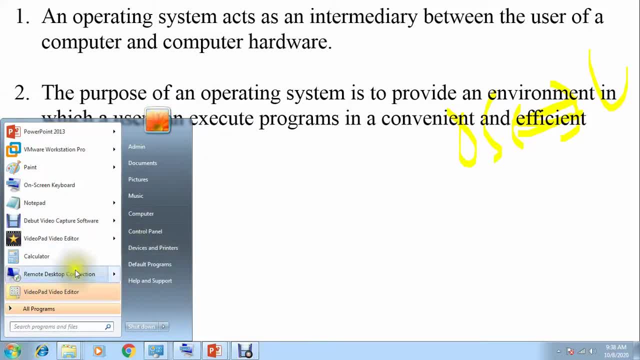 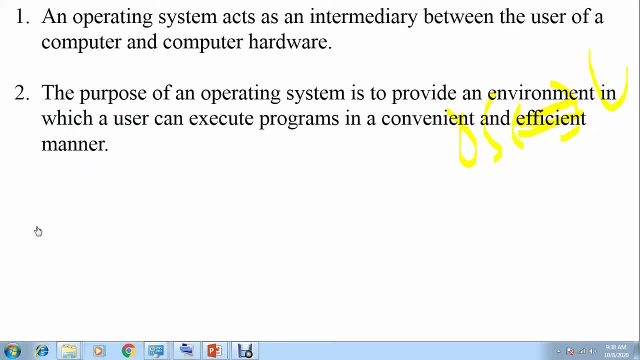 So if I want to access MS office, I can go to program. It is very easy, I do not need to do any extra thing and I can open anything like. if I want to open excel, it is very convenient to use. and if I want to go to control panel, I can go to control. 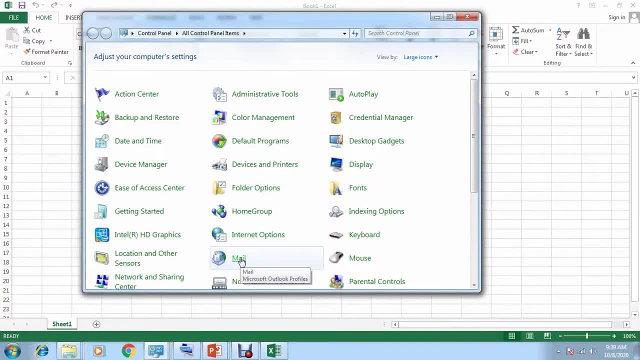 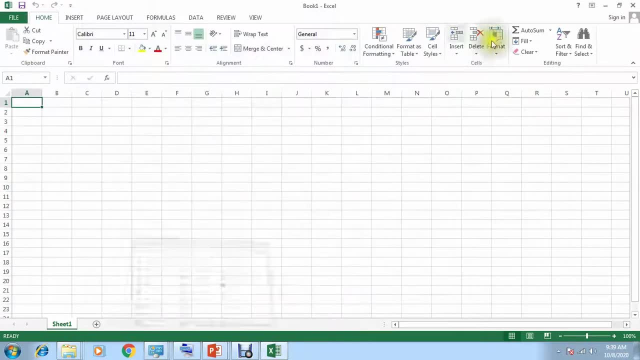 panel, I can do whatever I want to do. like you know, if I want to configure email, I can configure from here. It is very convenient and it is happening only because of operating system. Next, an operating system is a software that manages the computer hardware. 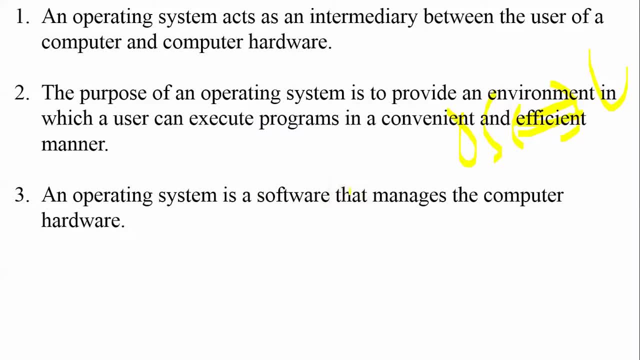 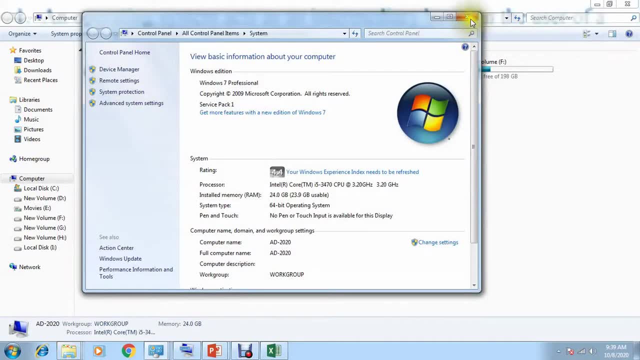 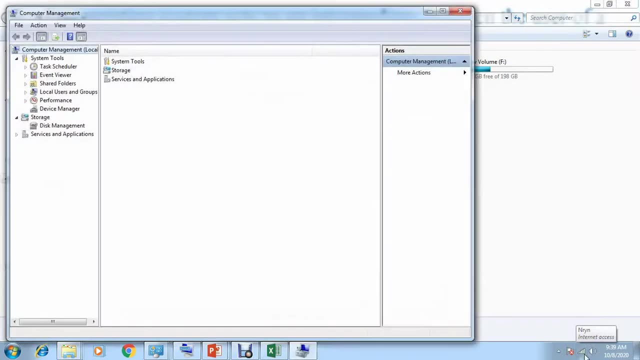 Yes, it manages computer hardware, For example. let me give you one example here. For example: here- sorry, I should go to manage here- For example: you can see: this is my Wi-Fi, I am connected to Wi-Fi. 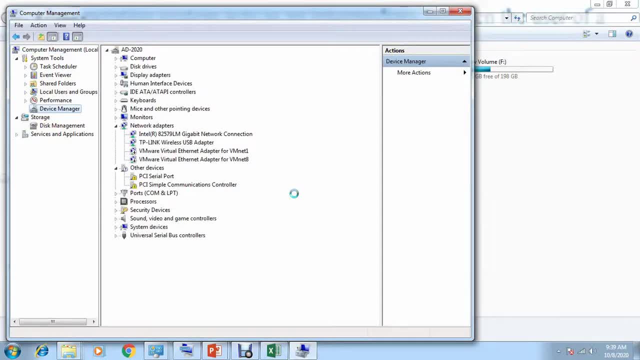 Okay, so Wi-Fi is like: until and unless we install driver, we cannot use any, any hardware. So I am using This is my desktop computer, so I have connected one adapter here. okay, wireless adapter. This is. I will show you here one wireless adapter I have connected. 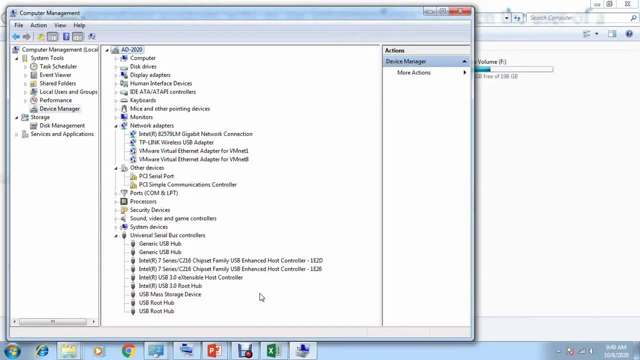 So that is I mean. then only I am able to use internet through Wi-Fi. So we need to install drivers and then only it will provide. you know, For example, this is LAN. If I don't install any driver for this, then I won't be able to see this, you know, LAN. 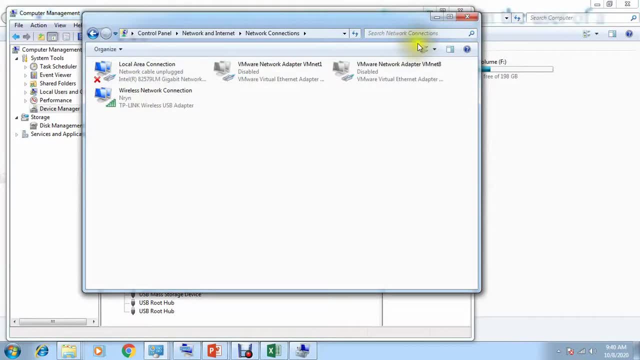 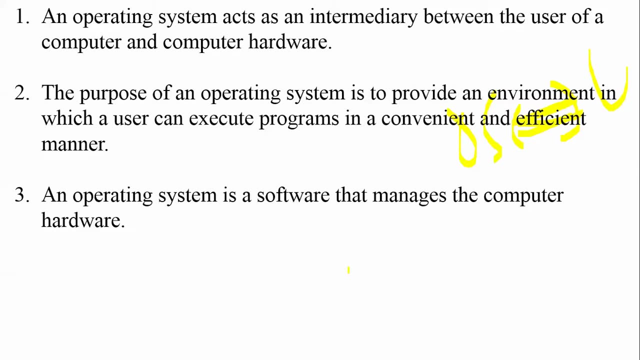 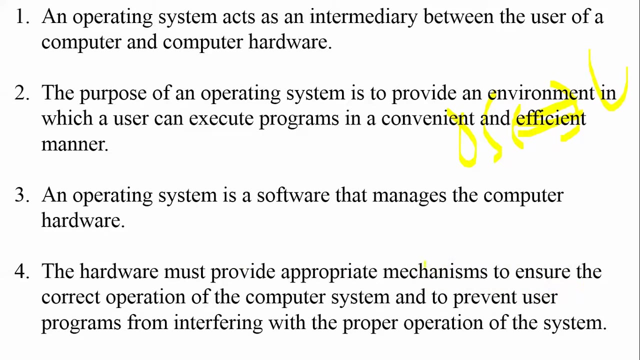 interface here, this. So that is what I mean to say here. An operating system is a software that manages the computer hardware, And the hardware must provide appropriate mechanism to ensure the correct operation of the computer system And to prevent user from you know user program. basically to prevent user program. 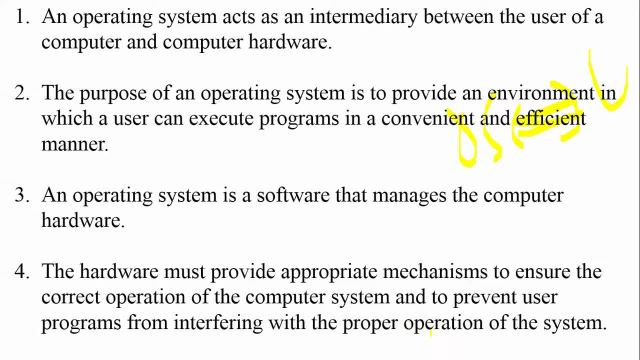 from interfering with the people proper in operation of the system. So the meaning is very simple: Whatever hardware is we are using here should perform- and you know should perform very well in a, in a proper manner where if I make any program, that should not prevent the operation. 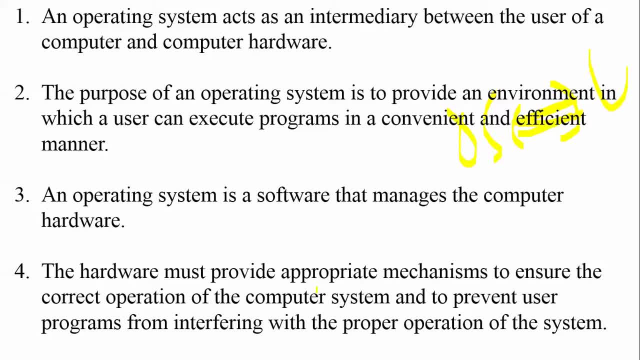 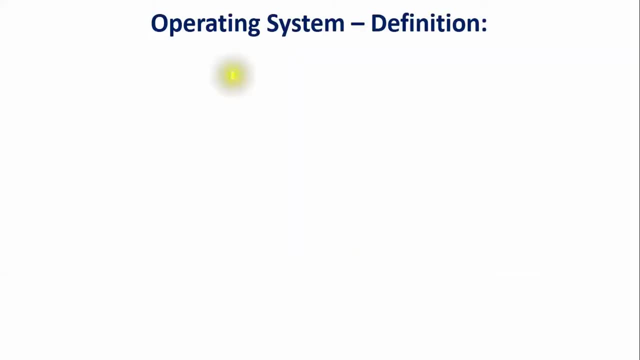 of operating system. If I make any change, it should not hamper, It should not impact the- I mean the proper operation of the computer hardware or operation of the system. And definitions. here there are lots of definitions available. You can go through Google and you can find thousands of you know definitions. 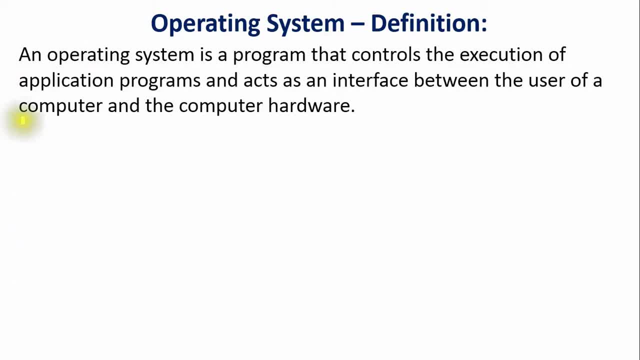 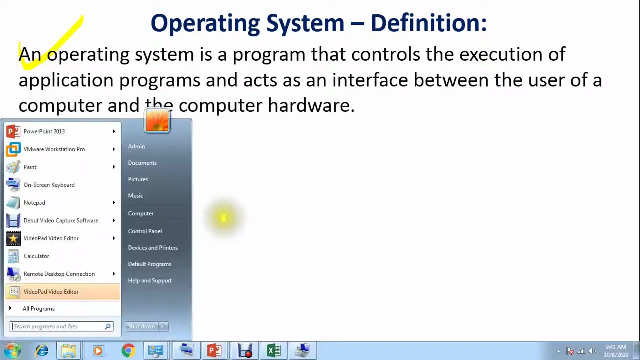 So here, one, one or two, two or three, I will be talking to you. So, guys, an operating system is a program that controls the execution of application programs And as an interface between the user of computer and the computer hardware. So the meaning is very simple. 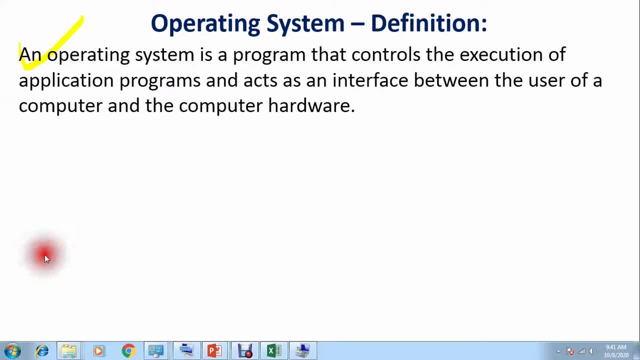 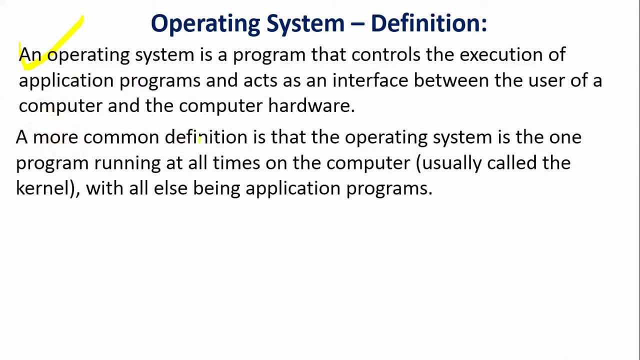 For example, if I want to open anything- calculator, or if I can go to a command from, from there also I can open calc. So it is helping me to execute programs Very simple, Okay, And so a more common definition is that the operating system is the one program running. 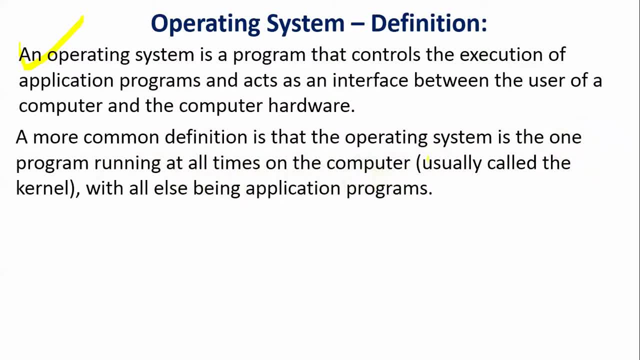 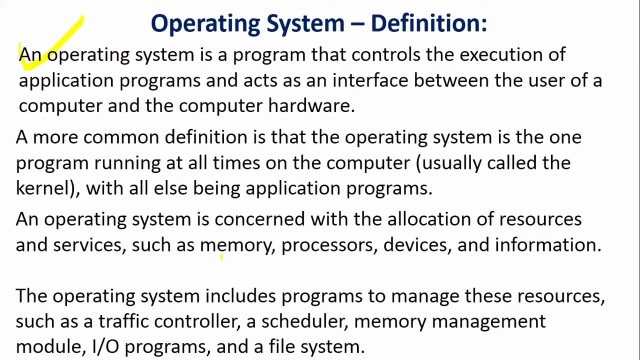 at all times on the computer, usually called a kernel, with all else being application programs And little more about it. An operating system is connected with the allocation of resources and services, such as memory processors, devices and information, And the operating system includes program to manage these resources, such as traffic. 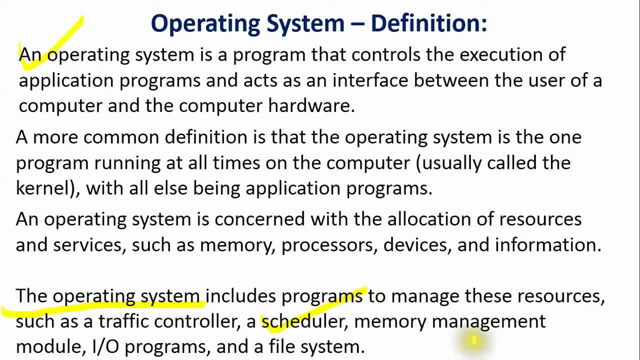 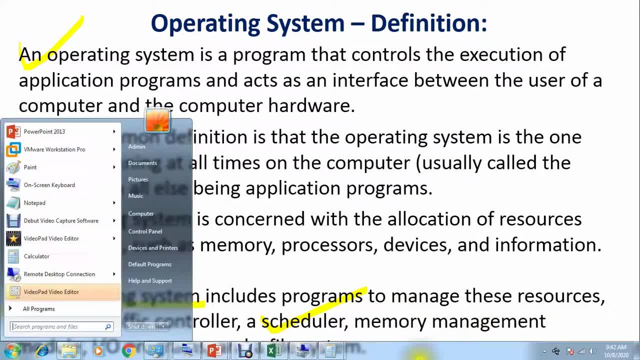 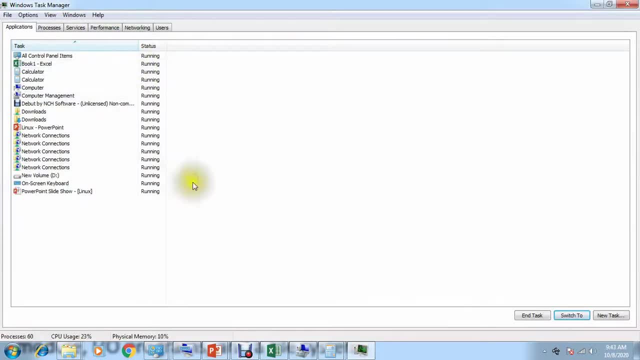 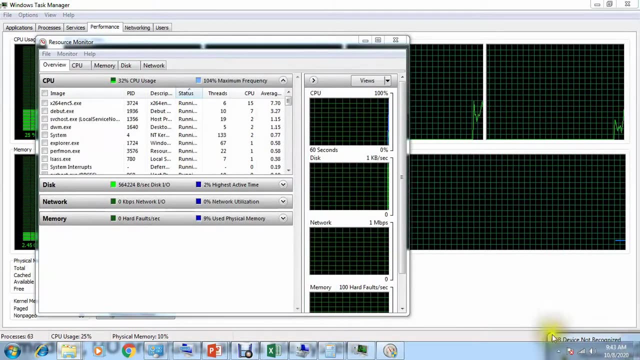 controller, a scheduler, memory management- Okay, And module input, output programs and file system. So what does it mean? Resource management means if you go to control panel you can see a performance and, like you know, go to performance here and resource management, you can see. all these things are. 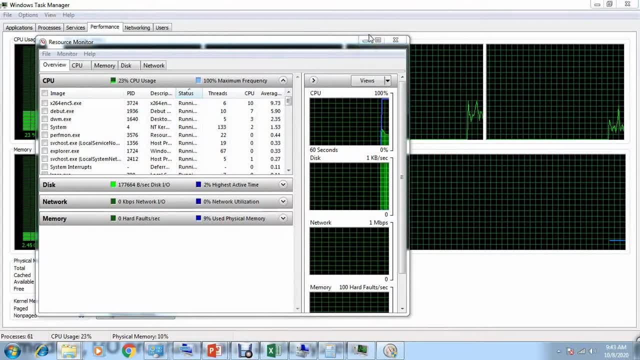 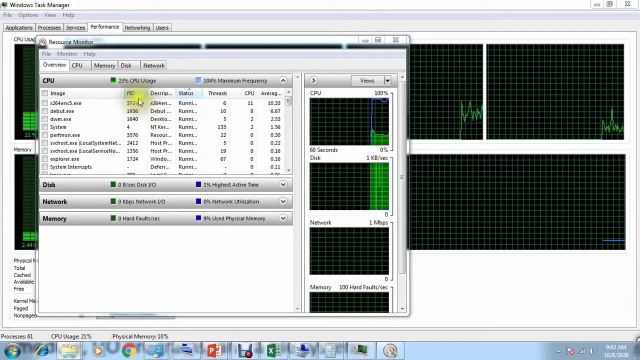 happening only because of operating system, and operating system is managing all those things Very, I mean, you know, in in very proper way. for example, you can see here memory utilization with all the uh by by all the uh process here. 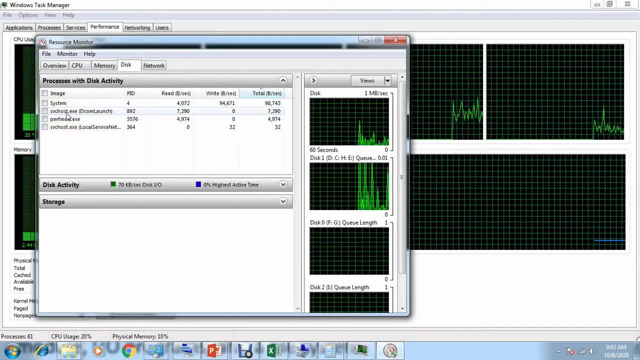 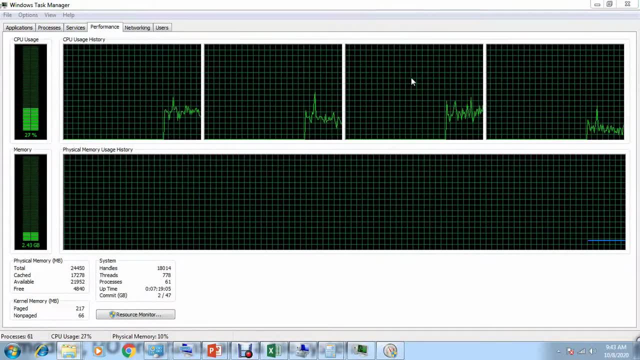 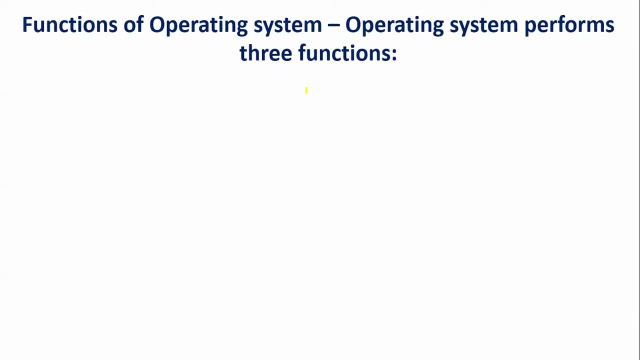 Okay, And even you can see a disk system. this couple of these are the process with disk activity running here. So it is happening only because of operating system. Now, function of operating system. so as operating system performs three functions basically. So one is, like you know, convenience. 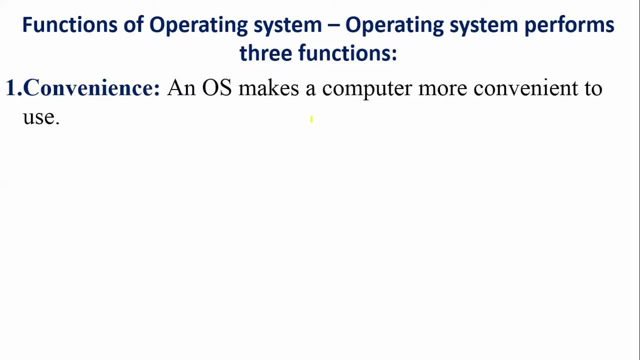 What does it mean Actually? an operating system makes a computer more convenient to use, very simple and, uh, efficiency. and operating system allows the computer system resources to be used in an efficient manner. What does it mean actually? So you can see here, so it is swing you. which process is swing you? I mean which process? 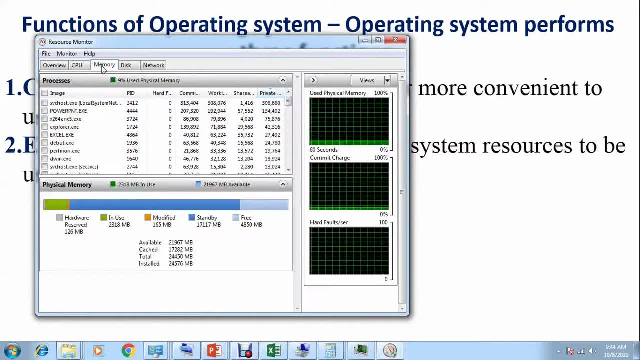 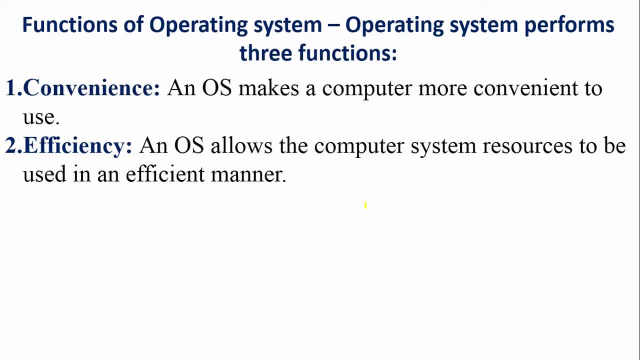 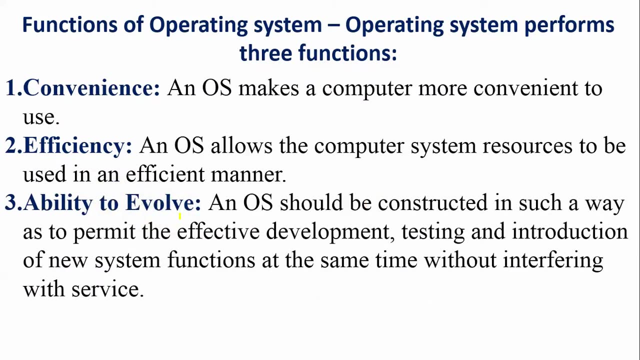 is using how much Ram, How much CPU? Uh, that is what it is telling you, and uh, and operating system allows the computer system resources to be used in an efficient manner. And the third one is a ability to evolve. So what does it mean actually? an operating system should be constructed in such a way. 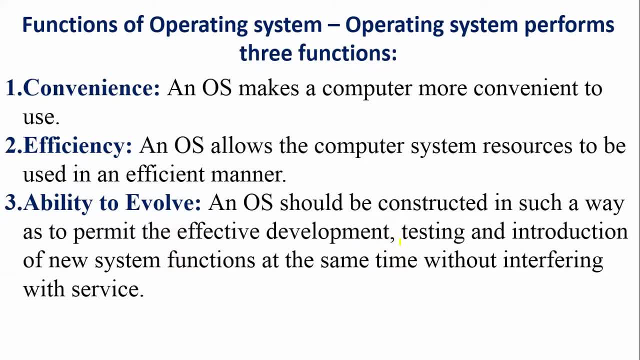 as to permit the efficient development, testing and introduction of new system functions at the same time. Okay, Now what it is. What is it supposed to mean? Well, the operating system has a different meaning with services, So meaning is very simple. 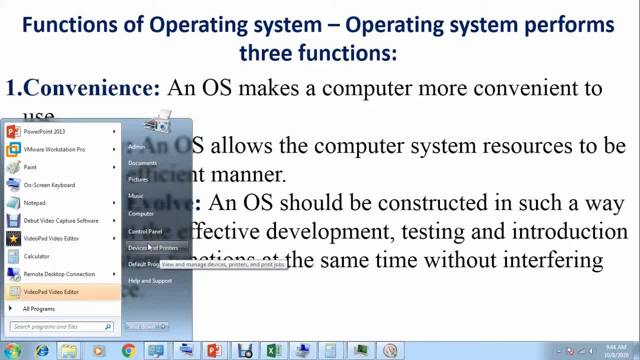 If I want to install 10,, 10 other uh you know- program like uh VLC player, apart from VLC player, Any other, if I want to install any game, if I have want to install any other program, so that should work properly, that should not impact any other service. 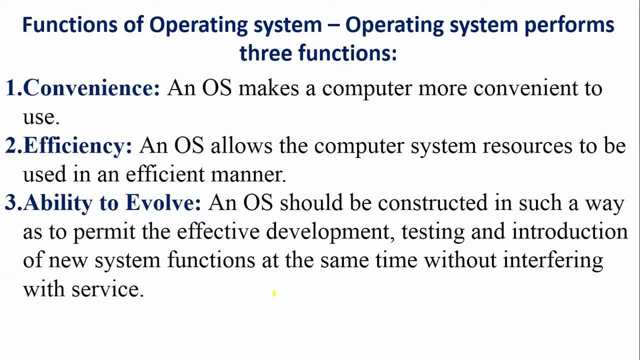 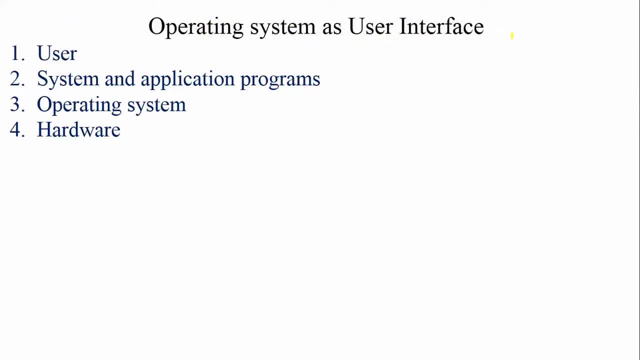 That is what, uh, it is telling you like: ability to evolve now this operating system as user interface. there are four layer basically in this operation, in this process. the first one is user, the second one is system and application program operating system, then hardware. let me show you what it is. 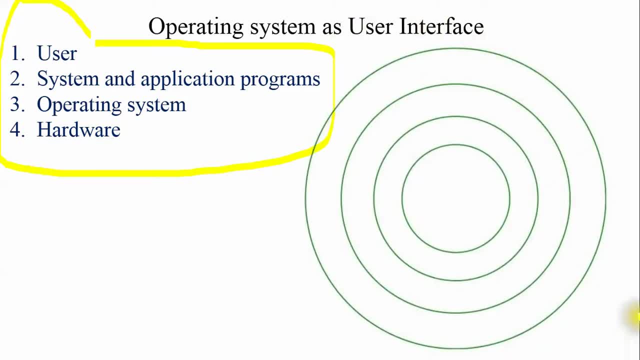 actually. so this is a life, i mean, this is a circle or this is, you can say structure or you can say, like you know, interface basically. so first one is here. i told you user, but user is and and number okay, and it comes in hand. so the very first one is hardware. what is hardware? your computer? 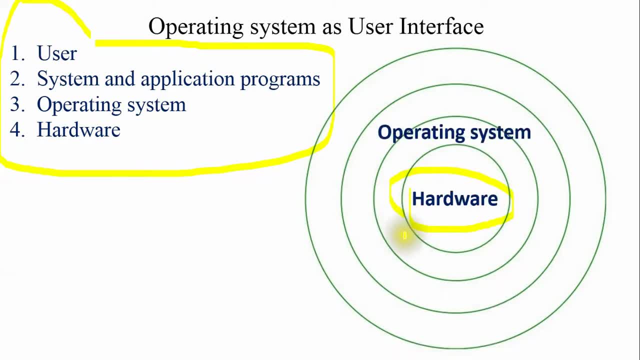 okay. second one is operating system. yes, operating system is a program, okay, and which controls which, which manages, which, allows hardware to function. and third one is system and application programs. there will be lots of applications will, i mean, will, be getting installed, uh, at the time of operating system installation by default. 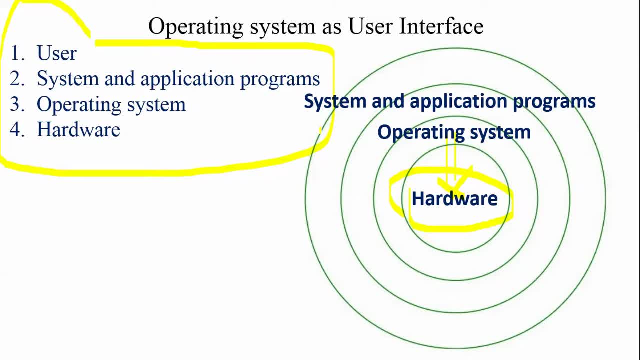 later on also, we can install some more. and the last one is user. user is going to use applications. applications will be running only because of operating system, and operating system is we. i mean operating system is going to be installed on hardware. so this is a complete interface where 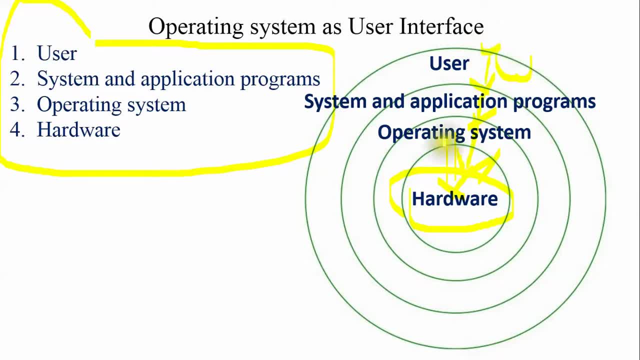 user is coming at the end. okay, if you don't have hardware, you cannot install operating system. if you are able to install operating system, you will have to purchase one hardware. then only you can use applications and programs. and who is going to use user? now i will tell you about little. 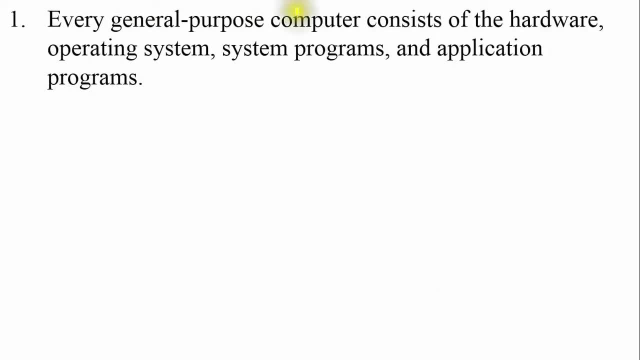 more. every general purpose computer consists of hardware. yes, operating system, computer program and application programs. very simple, for everything. you need these things if you are working on a computer or if you are doing any computer process. so you will have to use operating system program, a couple of things, for example, if i want to take print out. okay, so there, i should install some. 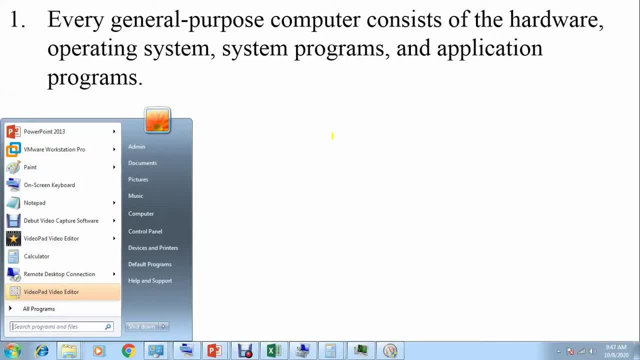 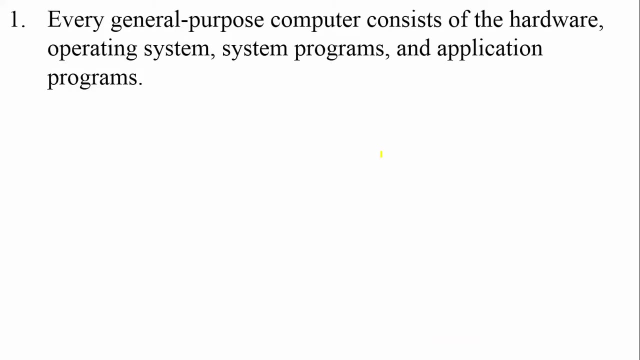 this thing. drivers and printer drivers we need to add, we need to attach to computer. okay and yes, we would require printer and that specific application for print and scan operating system, obviously, and the hardware consists of memory, cpu, alu and input output devices, peripheral devices and storage devices. 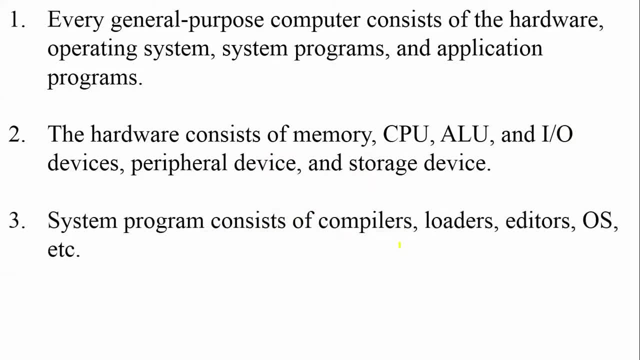 system program consists of compiler, loader, editor, os, etc. okay, yes, all these things will work together to make a system function properly and everything has certain specific role here. and the applications program consists of business programs, data, database programs, for example. guys, this is once again a conceptual view of this thing. just now, i 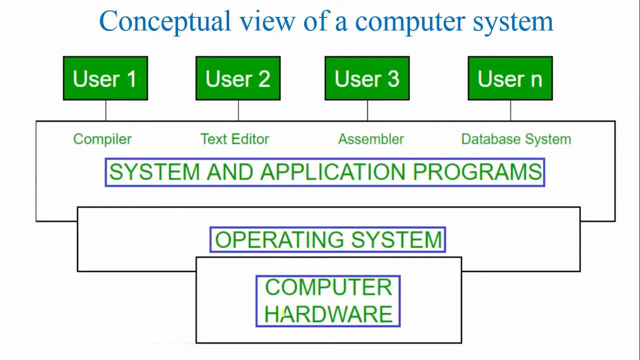 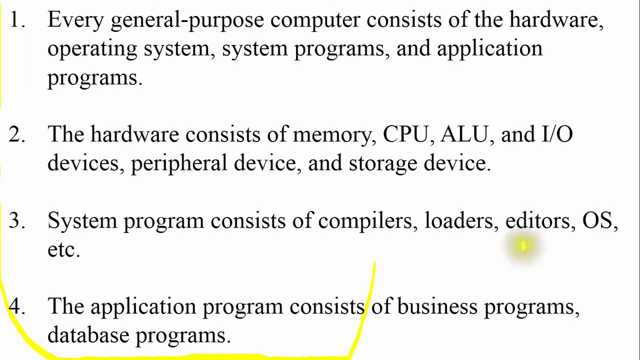 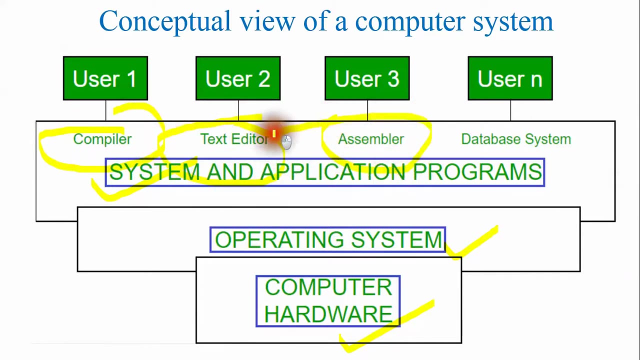 told you here what it is actually. so once again you got computer hardware, operating system system and application program. now here these things. just now i told you, like uh, system program consists of compilers, loaders, editor, operating system. so you will have one compiler, a text editor, assembler, database system, and here user can use one thing, you second can use second thing, third and 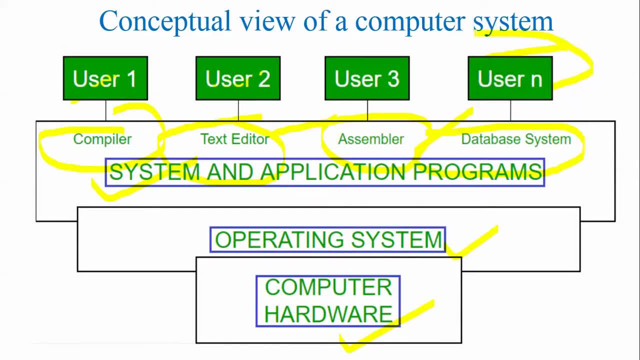 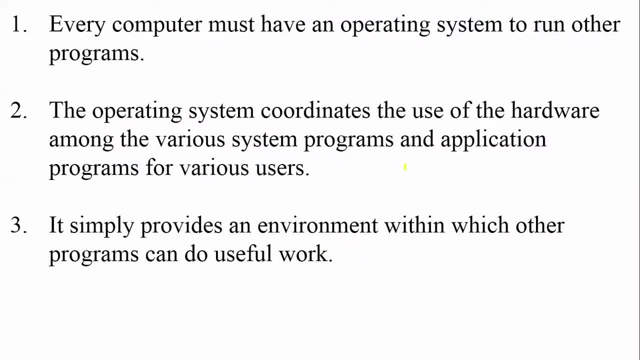 n number if users can use all those things as per the requirement. okay, so i will tell you here about compiler and assembler and in my coming up slide what it is actually. so, guys, here once again, like you know, same sort of stuff here. every computer must have an operating system to run the programs. 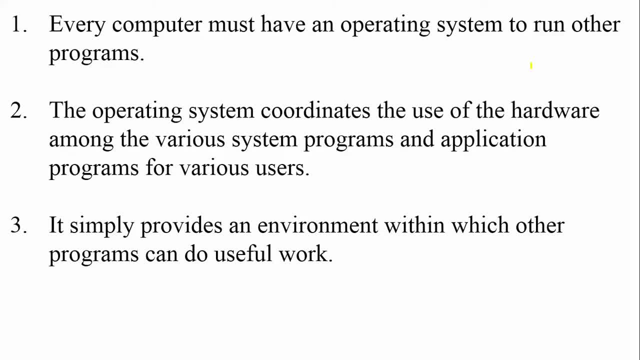 yes, obviously very simple. there should not be any doubt in this. if you want to run any operating, just any, any program, you need to install operating system. it can be any operating system open to linux or unix or windows, whatever, but you need operating system. and second thing, the 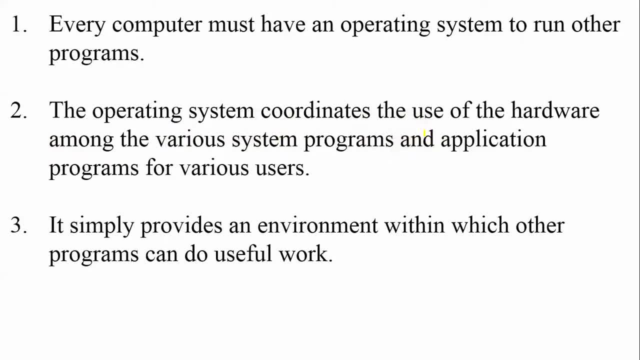 operating system coordinate the use of hardware among among the various system programs and application program for various users. it it simply provides an environment within which other program can do useful work, and the operating system is a set of a special program that run on a computer hardware that 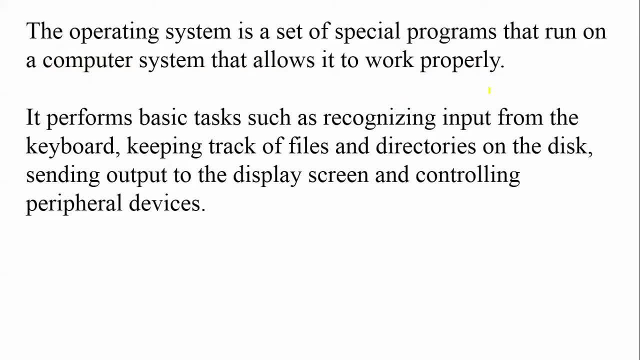 allows it to work properly. it performs basic tasks such as recognizing input from from the keyboard, keeping track of files and directories on the disk, sending output to the computer, to the display screen, and controlling peripheral devices. yes, whatever i'm doing, i'm doing only because of operating system. it is controlling each and everything. i am moving this mouse and i'm 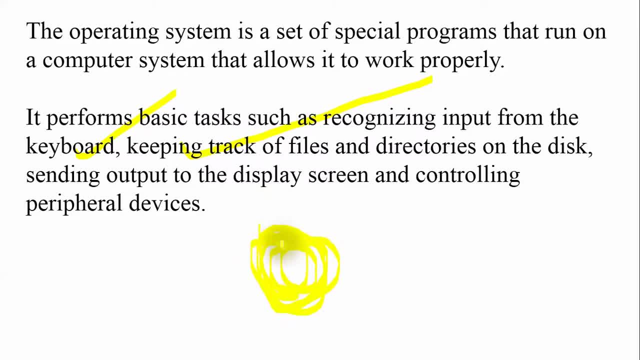 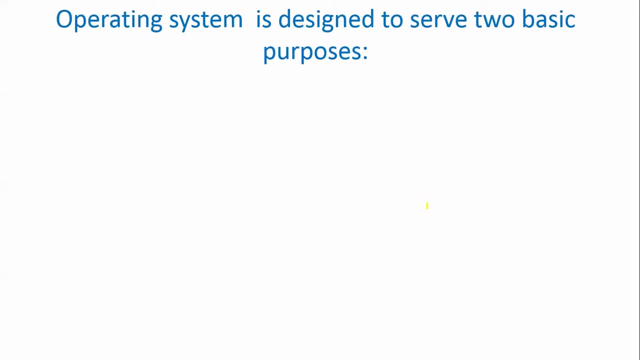 creating this circle, this kind of using this yellow color, okay, and it is displaying you here. it is only. it is coming only because of operating system and operating system is controlling all the devices like i have connected: usb mouse, usb keyboard. okay. now, operating system is designed to serve two basic purpose. there are two basic purpose to serve by. 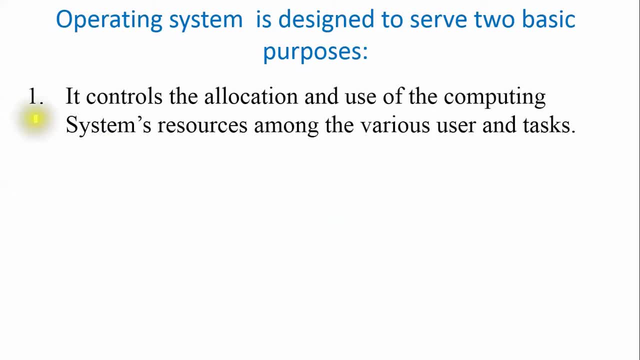 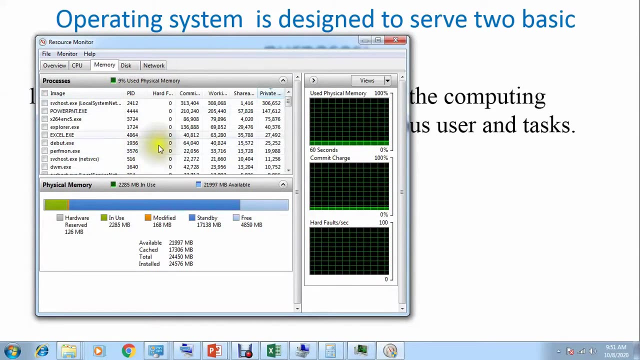 operating system. the first, the very first one, is it controls the allocation and use of the computing system resources among the various user and tasks. yes, just now i showed you here so it will give you complete detail about all the uh processes going on and how much resources they are consuming. 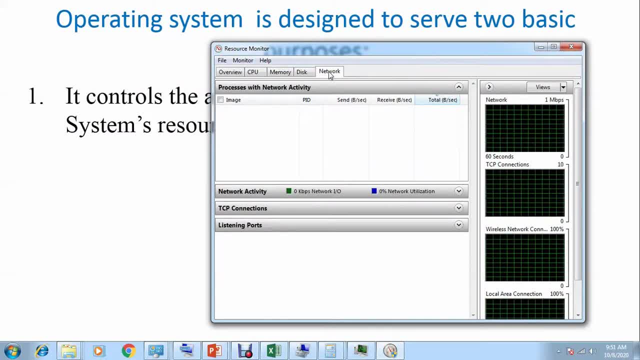 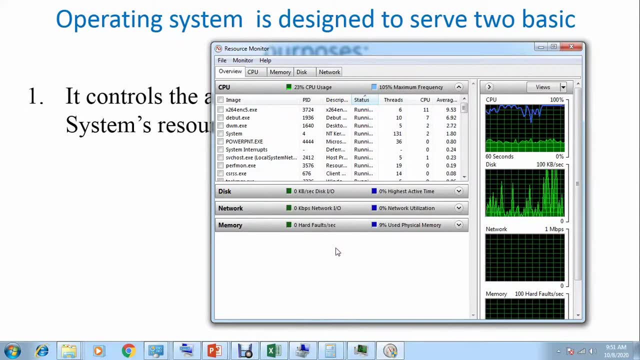 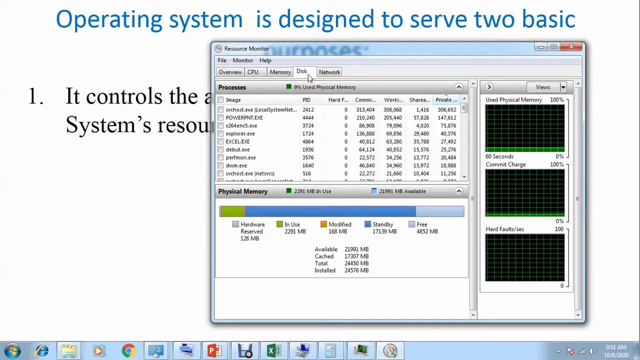 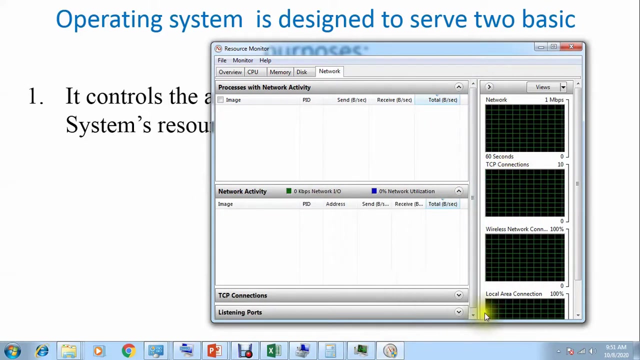 even. it will give you uh information about the user who is using uh as of now. i mean how much resources one user is using like that. so it gives you complete information and uh detail. okay, you can, you can expand it and you can see lots of things here and go little down. you can. 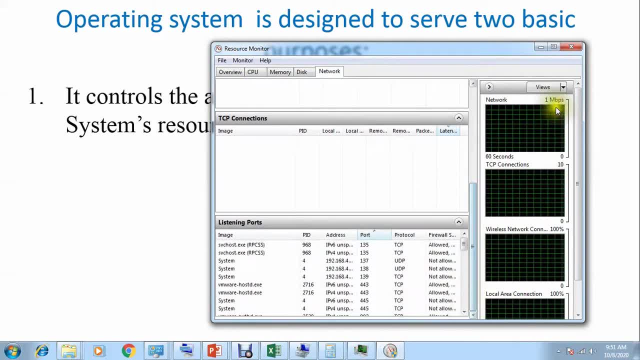 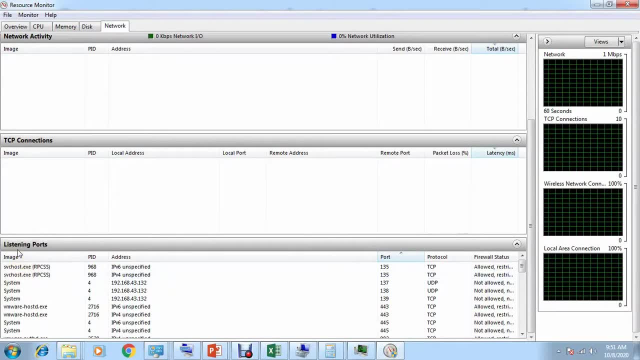 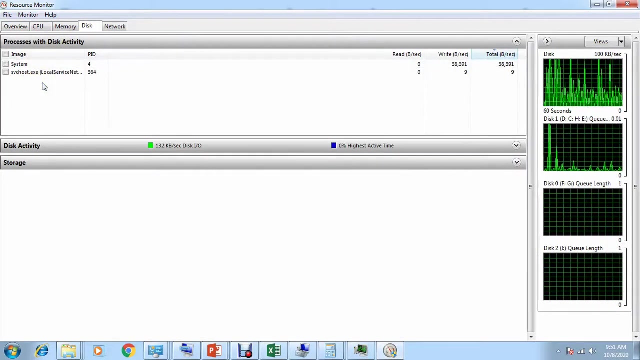 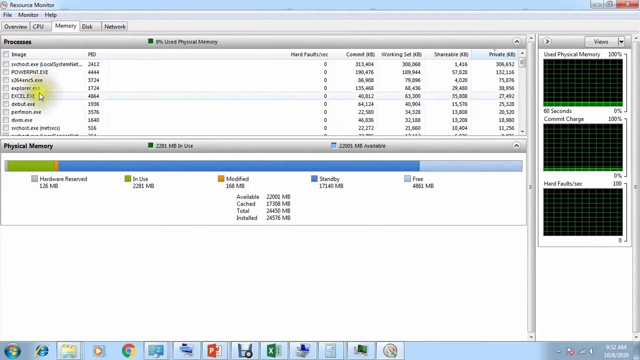 scroll it down, you can expand it. it is telling you like TCP connections, network connectivity, listening ports, and here you can see like network and once again wireless network connection, local LAN disk. you can see here image system. once again, here you can see memory utilization, CPU utilization overview. you can see here: 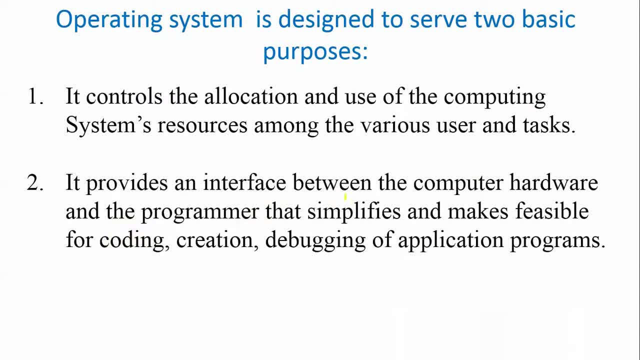 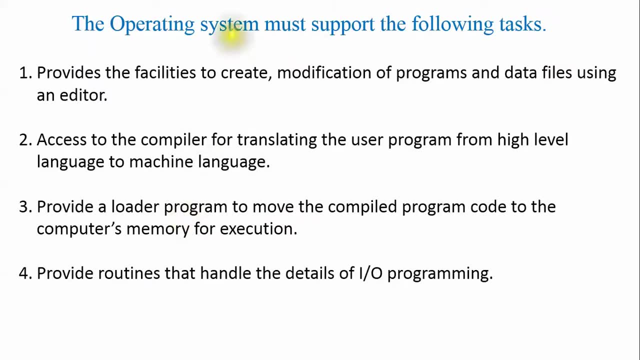 now it provides an interface between the computer hardware and program that simplifies and makes visible for coding, creation, debug, debugging of application programs. you can do it easily and, guys you know the operating system must support the following tasks but, for example, provides the facility to create modification of program and data files using an 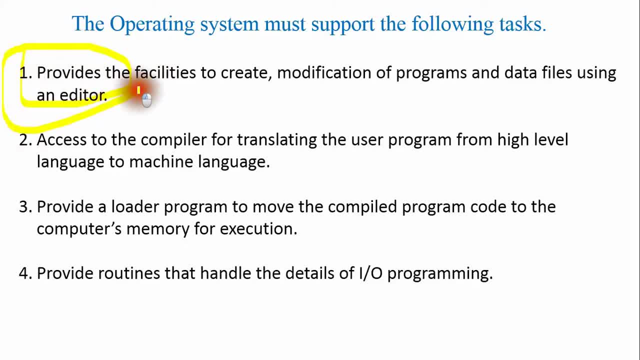 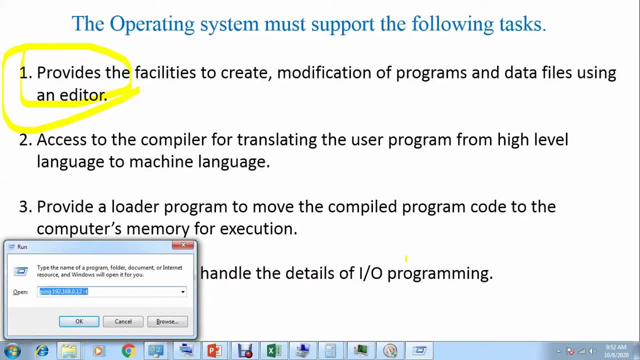 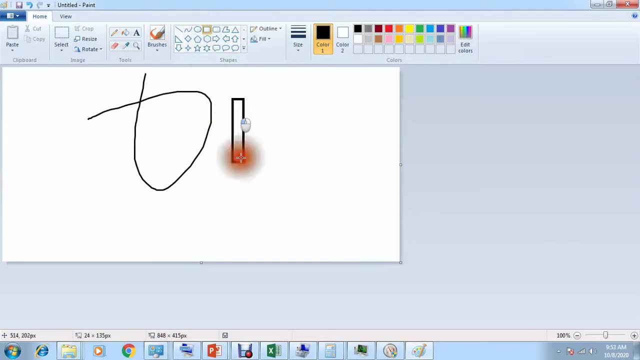 editor. that should be any editor. for example, I'm giving you well, for example, only I'm telling if I want to edit any image or how I should do it. I should have some editor. so this is, for example, MS Mint, I can edit this image- okay, and even I can create. so it should be. 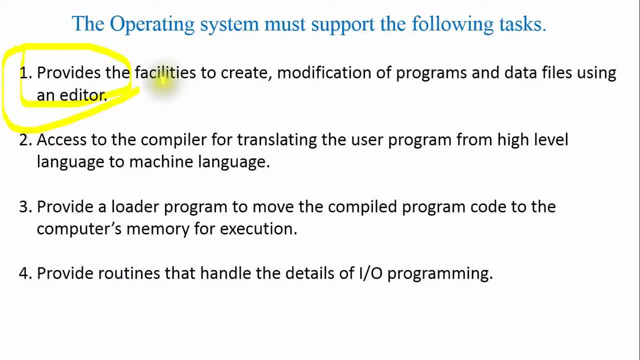 should provide that kind of facility first thing, and access to the compiler for translating the user program from being language to from high language to machine language. so meaning is very simple: if i want to create any software, my operating system should provide me that facility, because for that we will have to use- i mean- high level languages and provide a loader program to. 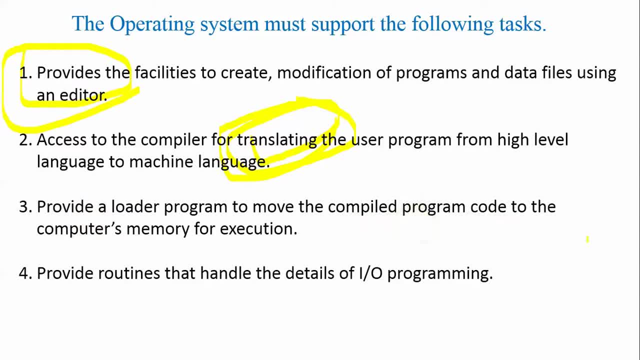 move the compiled program code to the computer's memory for execution. yes, loader, if you'll have one compiler, then loader. then i will tell you one more thing: provide routine that handle the details of input output, programs or programming. and what is input output? just a program or 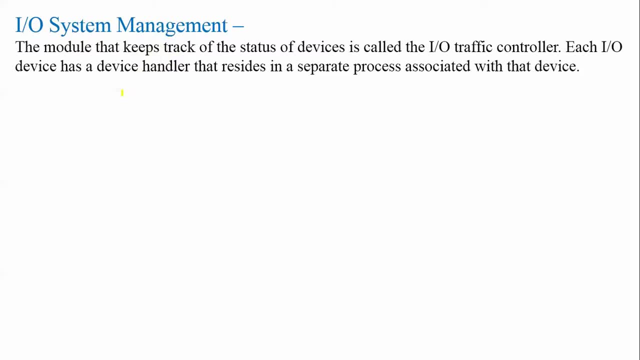 system. let me tell you here. so, guys, the module that keeps, that keeps track of the status of the computer's memory for execution- yes, loader, if you'll have one compiler, then loader, then i will. devices is called the input output traffic controller. okay, once again, i will tell you. 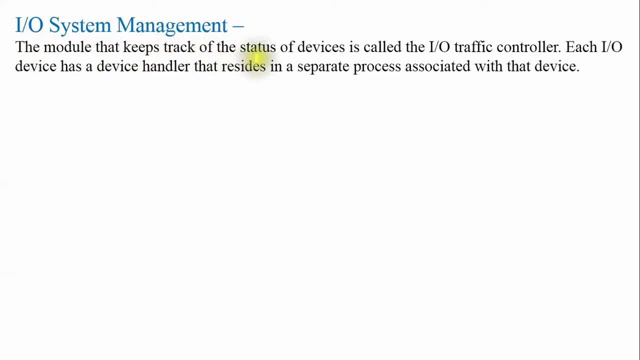 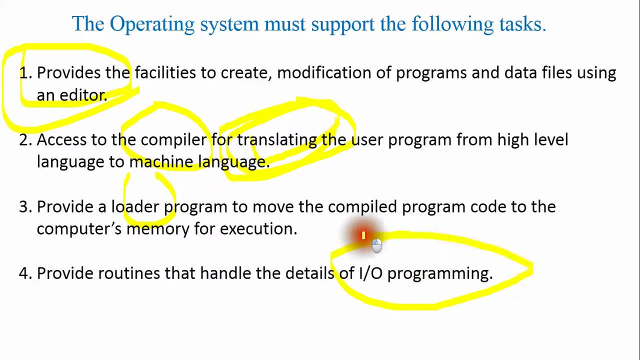 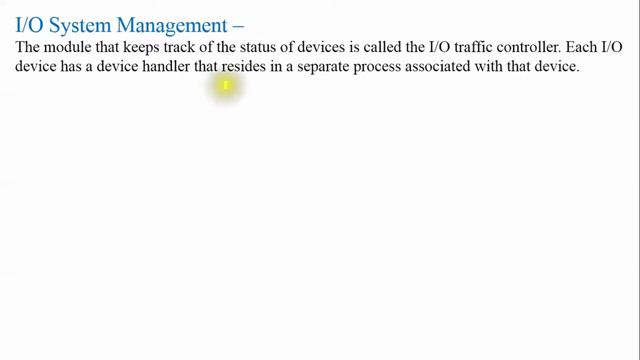 the module that keeps track of the status of devices is called input output traffic controller. i'm talking about input output programming or input output management system. so each input output device has the device handler that resides in the separate process associated with that device. and here the input output subsystem consists of a memory management component that includes: 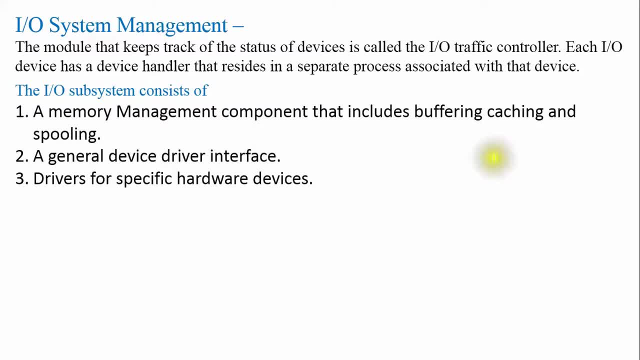 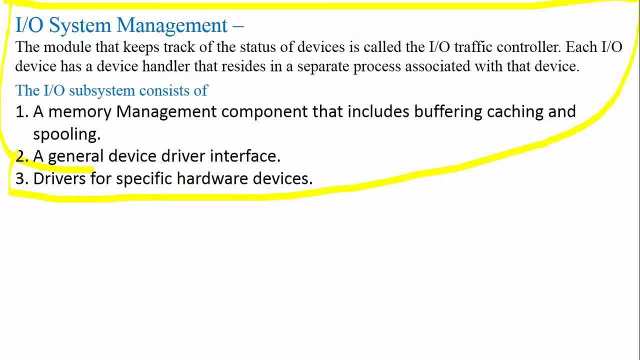 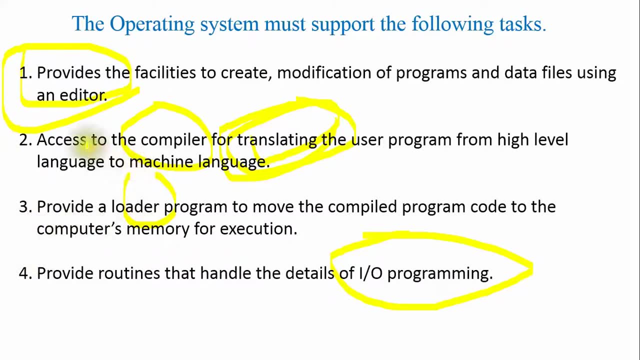 known as input output system management. and here i will tell you about assembler, because we spoke about a couple of things here, like you know: uh, access to compiler from uh for translating the user program. so what it is actually compiler, now i will tell you here so you can see here it is. 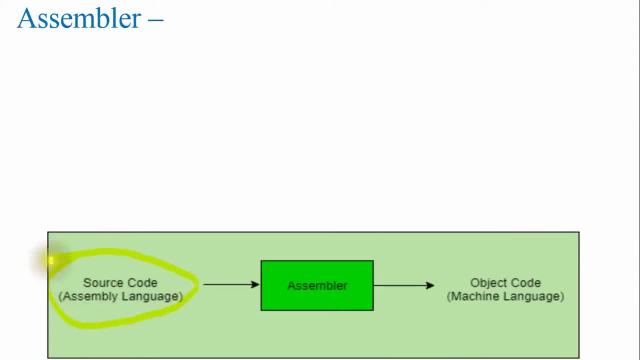 telling you source code assembly language, it is going to assembler and object code machine language. so let me introduce you about it. so, guys, the input to an assembler is an assembly language program. okay, very simple like this: source source code is assembly language, the output is an object program. 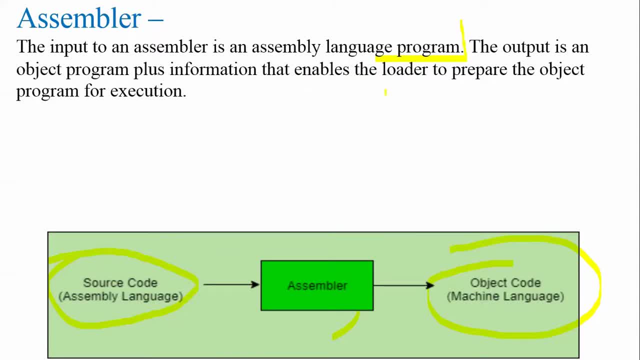 plus information that enables the loader to prepare the object program for execution. so it is a plus two. it is a combination of two things okay. one is the output is an object program, plus it is an object point. okay, so if in case the button close, it is because if you have a performing environment, if the counterpoint it has a��. 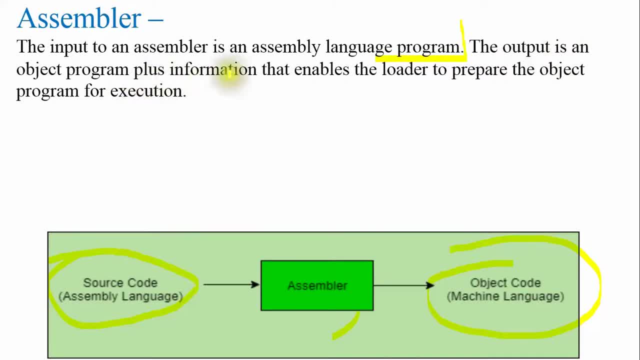 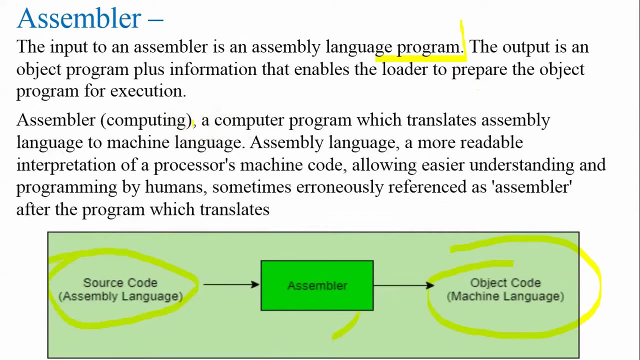 object program plus. so whatever is coming that after the process, that plus information that enable the loader to prepare the object from program for execution. and once again I will tell you where, assembler in computing, our computing, I will tell you: assembler, a computer, computer program which translates assembly language to machine language and assembly language a more. 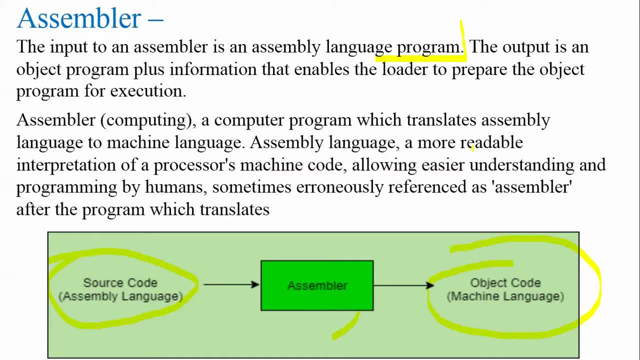 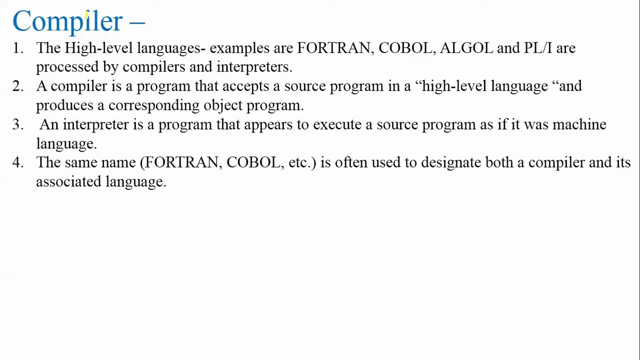 readable interpretation of a process, processor, machine code allowing is the easier understanding and programming by humans. sometimes the errors me erroneously report as assembler after program, which translate now compiler, we will talk about compiler. so the high-level language example for trends, COBOL, ALGOL and PL, this kind of 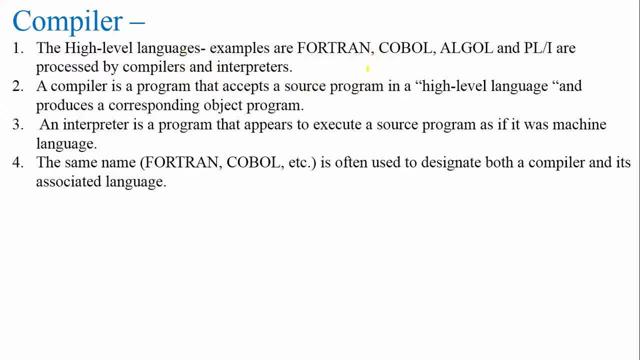 these are the very high level language and are processed by compiler and interpreters. so an compiler compiler is a program that except a source program in high language and produce corresponding object program. an interpreter is a program that appear to execute a source program as if it was machine language and the same name, like 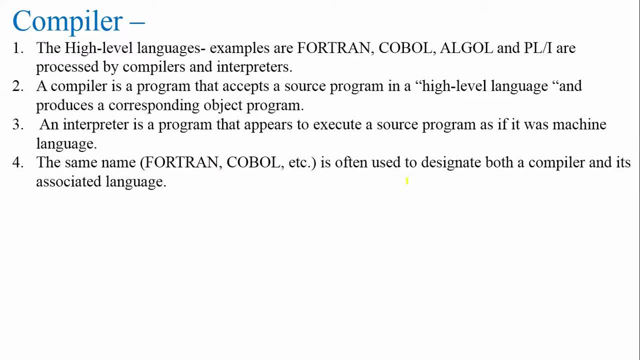 Fortran, COBOL, etc. is often used to designate both compiler and its associated language. so this is example. we will be using high-level languages. then compiler will come here and compilation errors- if any errors- that it will tell you: yeah, there is a error, and then it will convert it to. 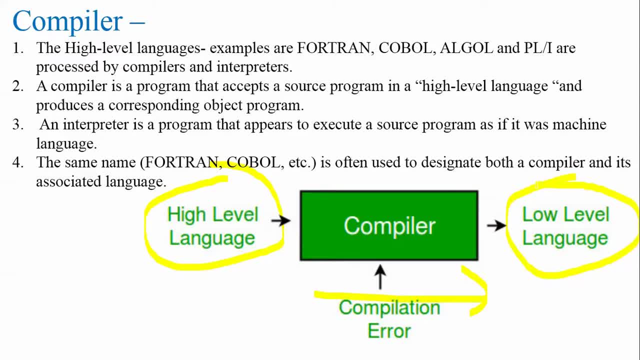 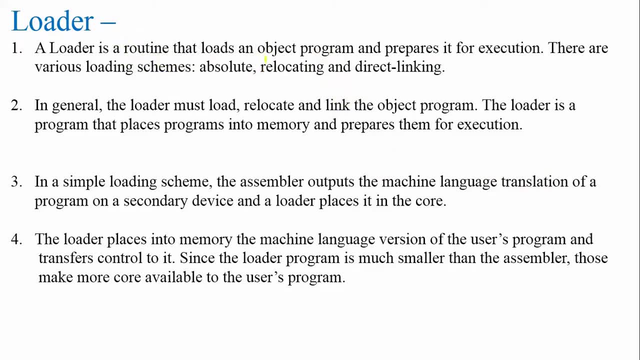 low-level language. next thing. next thing is loader here okay. so, guys, a loader is a routine that loves an object program and prepare it for execution. there are various loading scheme: absolute loader, relocating and direct linking. so, guys, you, you doing, you know engineering in computer science, then you will learn. 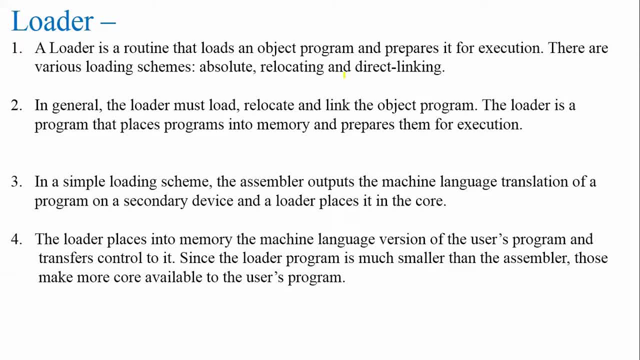 about it in detail because there will be separate- you know, chapter separate- book about all the languages, all those things, how it is actually in, how it works and in general the loader must load, relocate and link the object program. the loader is a program that places program into memory and prepare them for execution. so 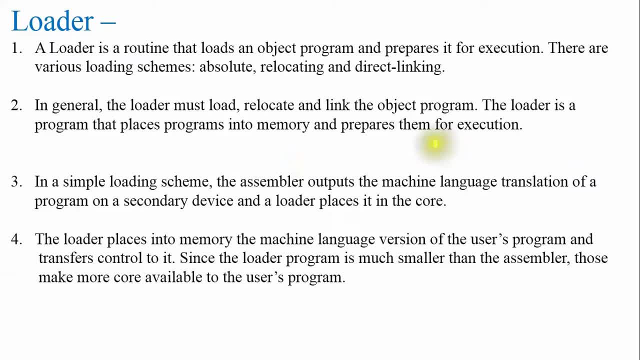 loader is, like you know, it is a final stage in this. in a simple loading scheme, the assembler outputs the machine language translation of a program or a secondary device and a loader places it in the code, and the loader places this loader into memory and prepare them for execution. 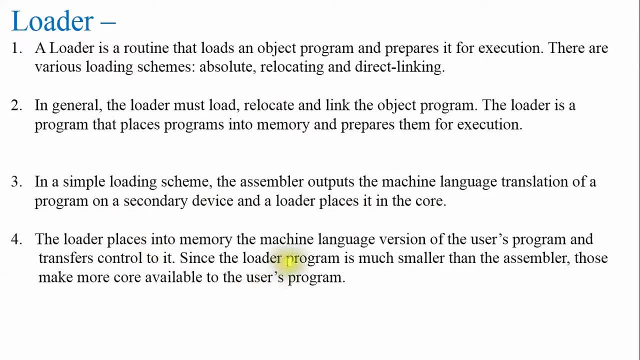 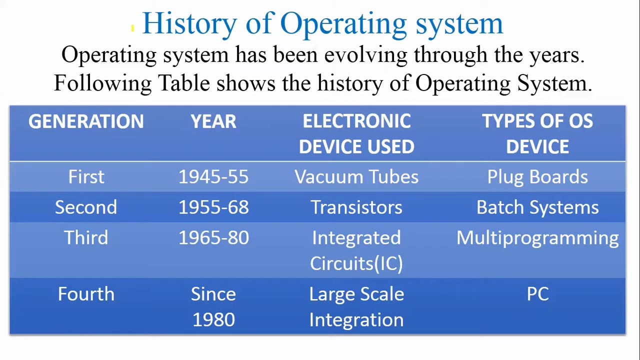 places into memory the machine language version of the user's program and transfer control it to it. since the loader program is much smaller than the assembler, those make more core available to the user's program. and now we will talk about sorry guys, about history of operating system. 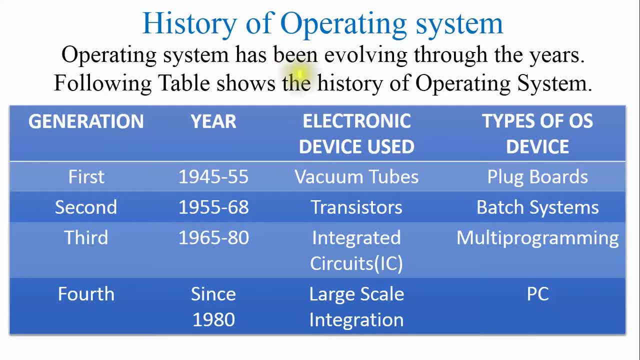 so, guys, operating system has been evolving through the years. from this table you can see here: okay, this is generation, this is year and electronic device used, type of device. so the very first is like 1945 to 1955 and the used device was vacuum tubes and type of operating system. 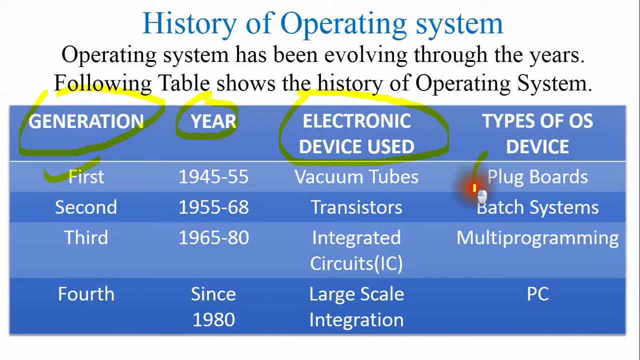 device was used like plug plug plug boards, okay. and the second one is 1995. this was 1945 to 55 and this is 1955 to 68. so they used transistors, okay, and this was batch system. and the third one is 1965 to 80, integrated chip. 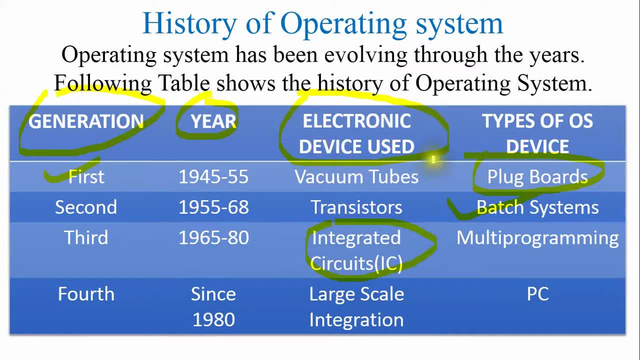 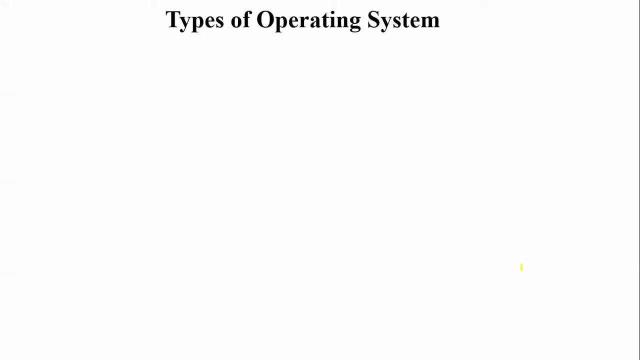 as electronic device used, and this was multi-programming operating system. type of OS device: okay. and fourth is, since 1980, largest scale integration, which is personal computer. okay, so now we are using at present personal computer only and largest scale integration operating operating system. now, guys, I will tell you about types of operating system. so there are. 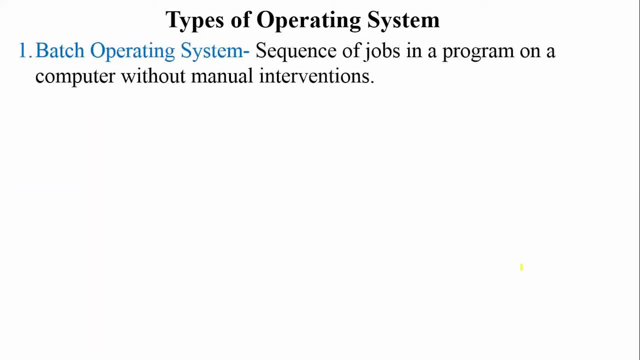 lots of operating system, types of operating system, types of operating system. types of operating system. okay, we should know about it. the very first one is vast operating system, batch operating system. so, guys, I will, I will try to give you detail about all the operating system, types of operating system. 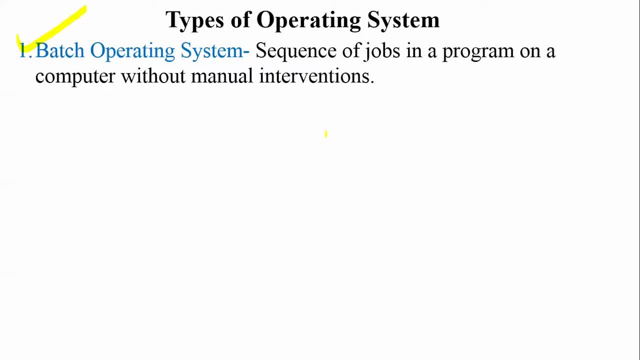 in my coming up videos and here I am just giving you a small intro. so what? it is actually a batch operating system saying this was used in second generation. okay, project that system. you know we. So what happens here? Sequence of jobs in a program on a computer without manual interventions. 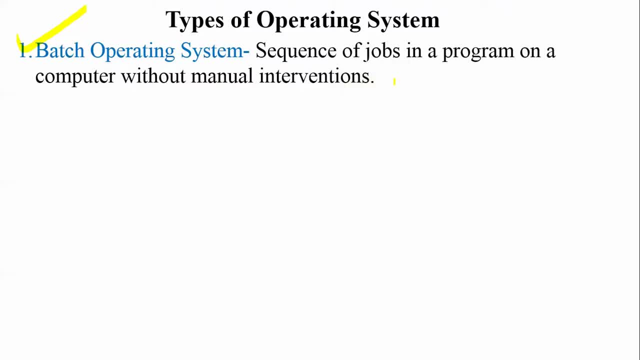 So here there was very less manual intervention, Okay, And the job was placed in sequence in a program. Second one is time sharing operating system. So it allows many users to share the computer resources, maximum utilization of the resources. That is known as time sharing operating system. 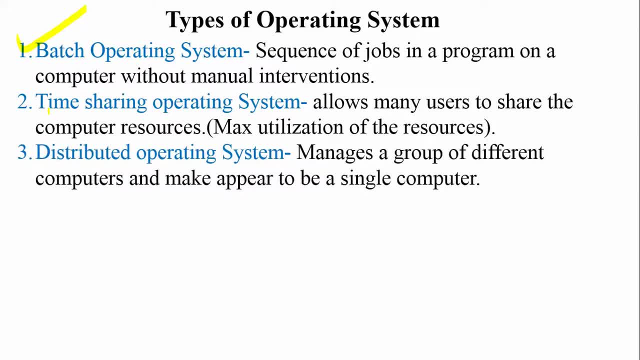 Third one is distributed operating system. So it manages a group of different computers and make appears to be a single computer. That is known as distributed operating system. Fourth one is network operating system. So, guys, network operating System, like computers running in different operating system can participate in common network. 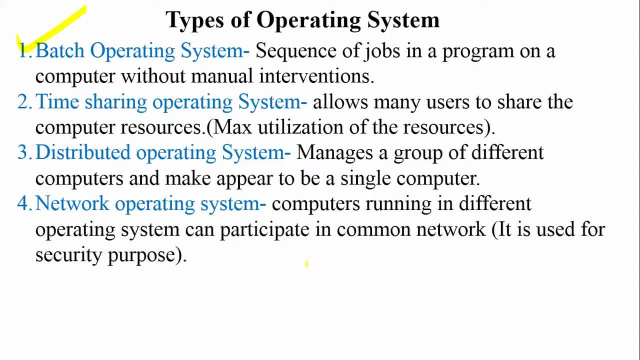 It is used for security purpose. Next one is real-time operating system. They are meant applications to fix the deadlines. So, guys, these are the you know types of operating system. in my coming up video and one of video, Definitely I will be speaking about detail.